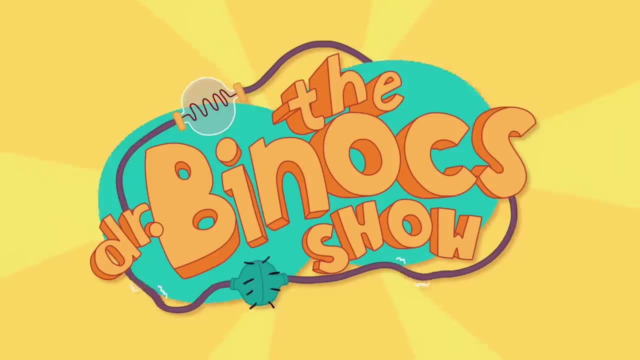 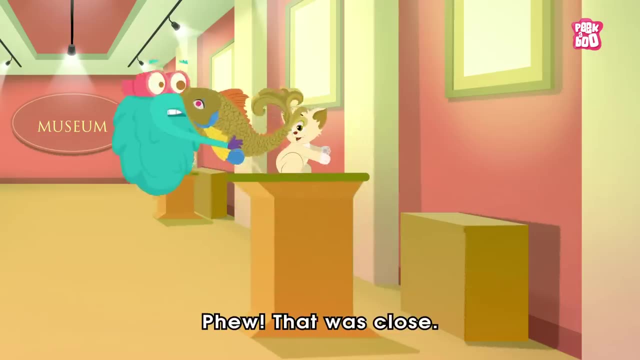 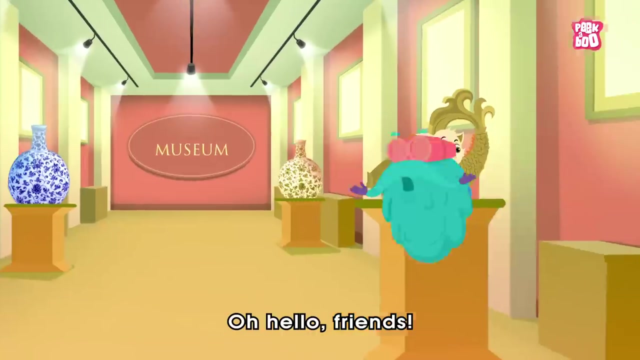 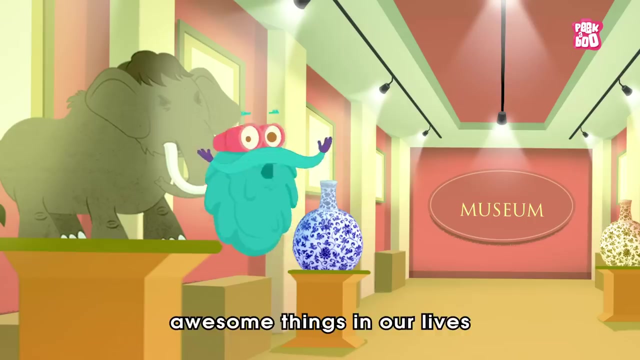 Oh no, That was close. Thank you, doctor. Oh no, little kitty, Don't thank me. Instead, thanks to my brain. Oh, hello friends. Yes, you heard it right: The reason we can do all these awesome things in our lives is due to an essential organ in our body called the brain. 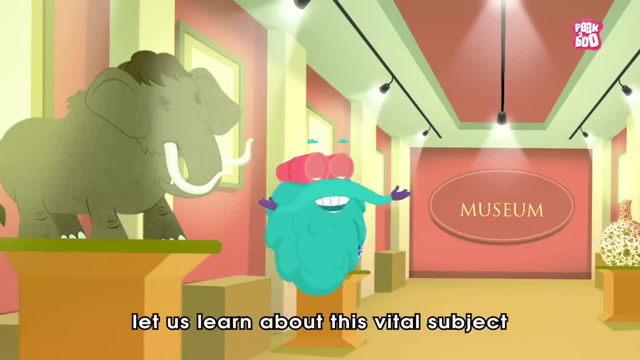 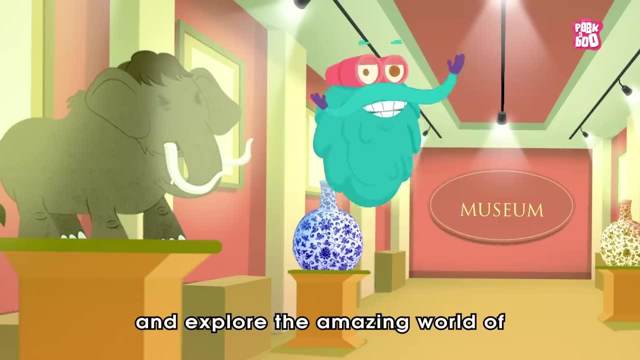 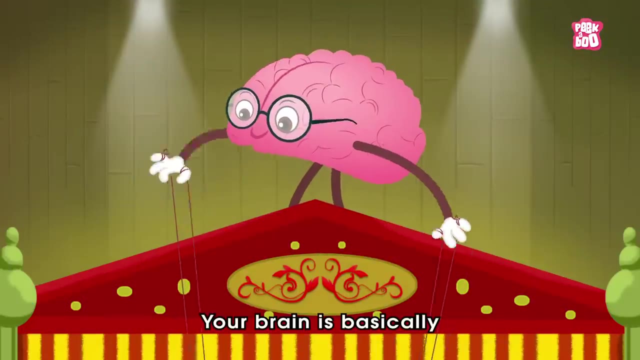 So today, let us learn about this vital subject that helps us to learn about the vital subjects And explore the amazing world of the brain. Zoom in: Your brain is basically the brain, The boss of your body, as it controls everything you do. 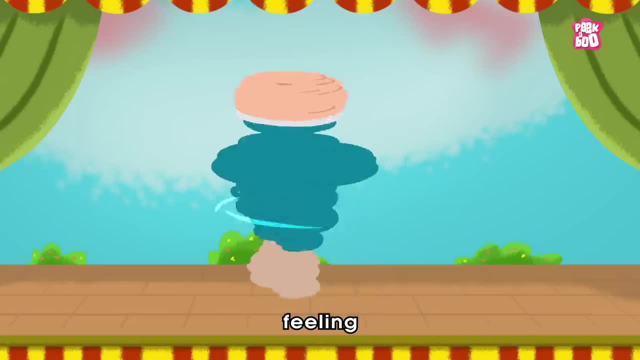 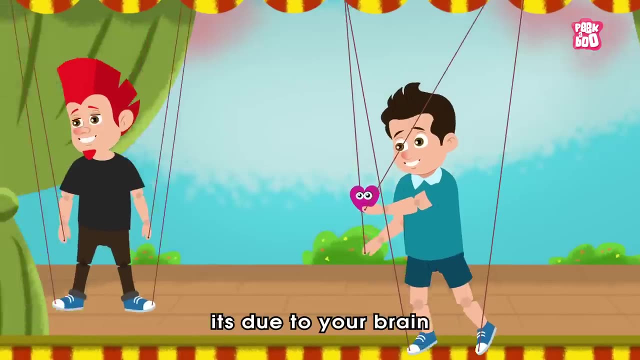 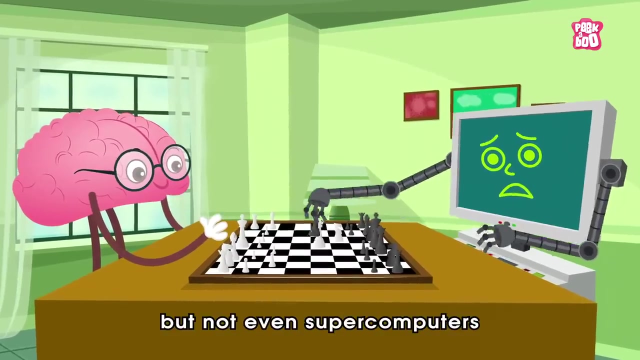 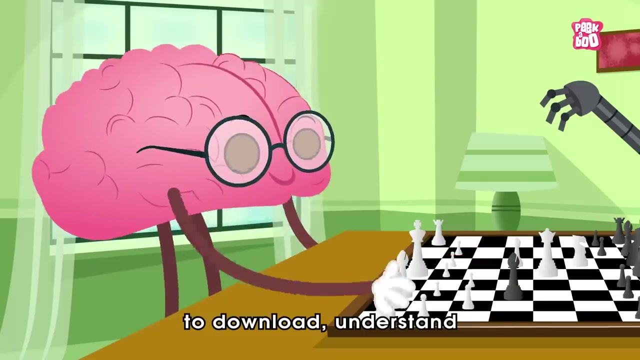 Things like learning, thinking, feeling, dancing, even breathing and your heart rate. It's due to your brain. you can pull pranks on your siblings and friends And you won't believe, but not even super computers can match its powerful ability to download, understand. 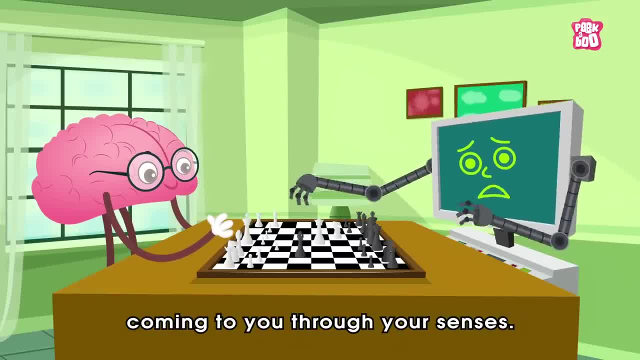 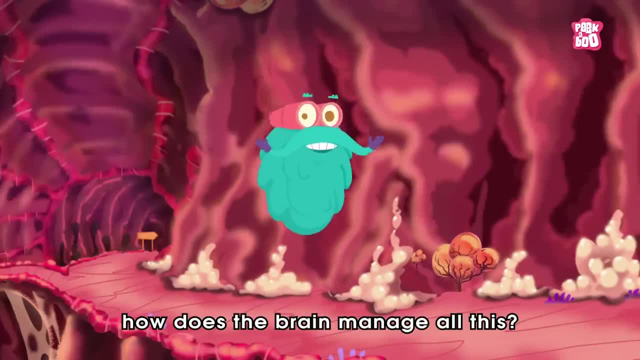 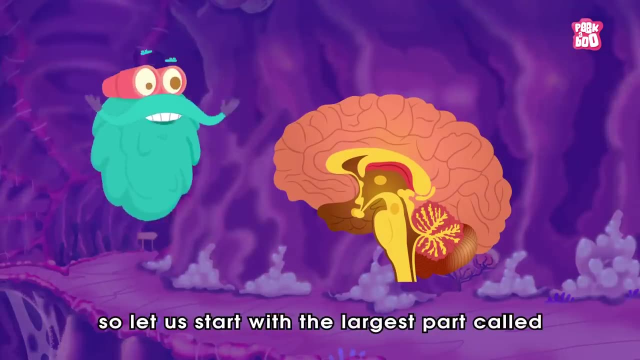 and react to the volume of information coming to you through your senses. So how does the brain manage all this? Different parts of your brain control different functions, So let us start with the largest part, called the cerebrum. that takes up to 85% of your brain. 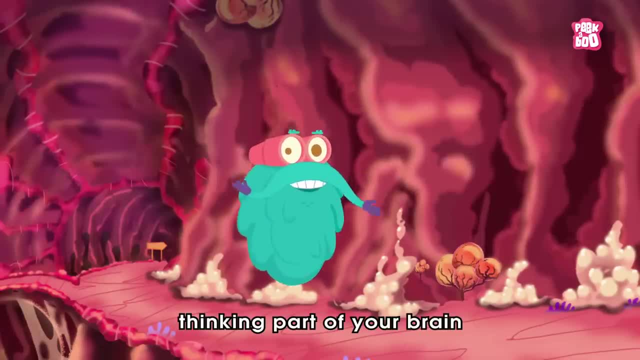 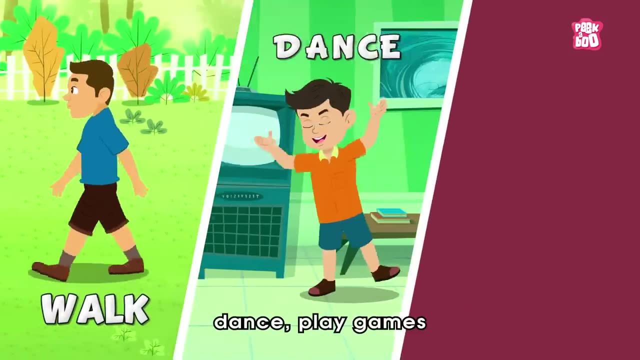 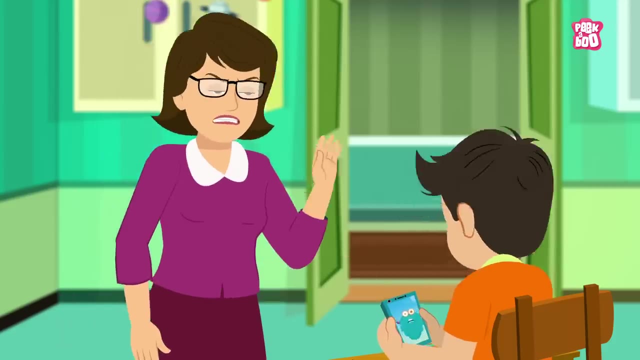 It's actually the thinking part of your brain and controls your mind. It's due to the cerebrum. you can walk, dance, play games and, most importantly, learn about various subjects on The Dr Binoc Show. Isn't it cool, friends? 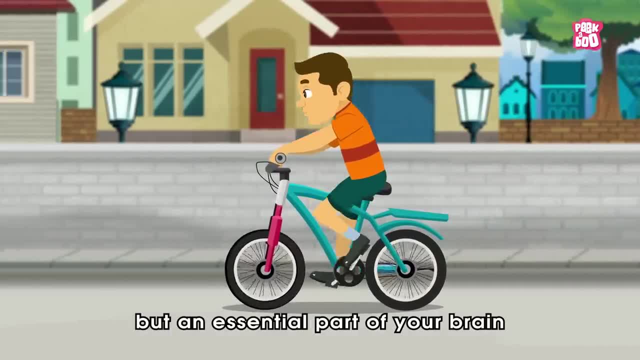 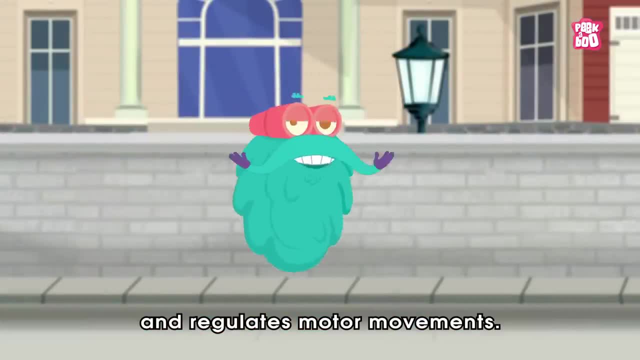 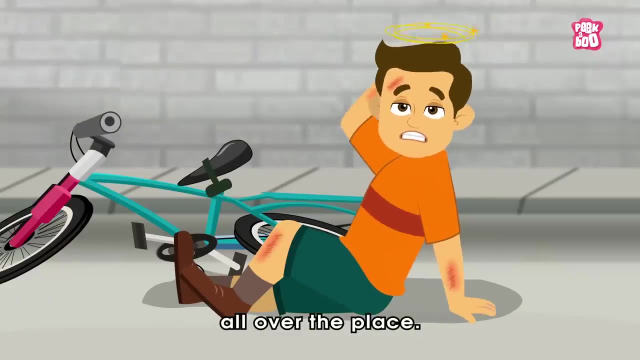 Next comes a relatively small portion but an essential part of your brain called the cerebellum, Which helps you to maintain your balance and regulates motor movement. That means, without the cerebellum you would be falling all over the place. Now comes a small but a mighty force to be reckoned with.